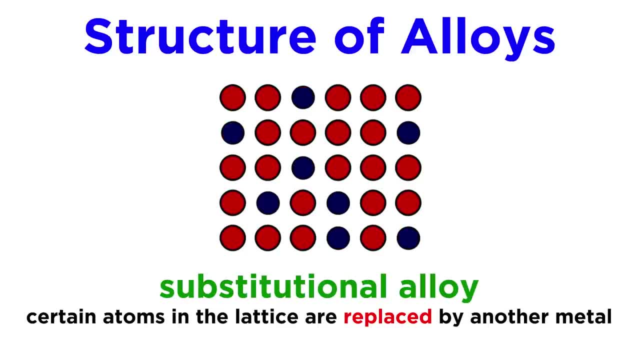 Substitutional alloy is one in which certain atoms in the lattice are replaced by atoms of some other metallic element. So, as we can see, atoms of one element are replaced by atoms of another element at certain positions in the lattice. This is a common structural arrangement when the metal atoms are of roughly the same size. 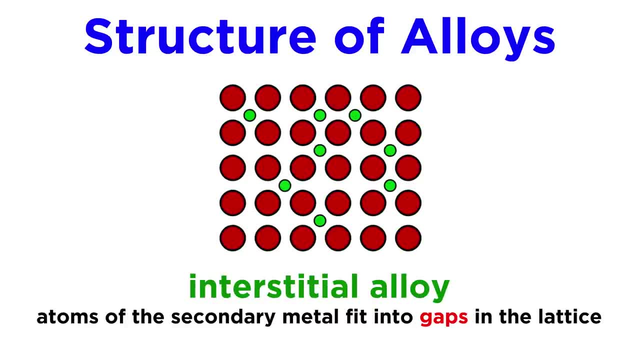 An interstitial alloy is one in which the lattice comprised of the primary metal is intact and atoms of the other metallic element can be found at certain interstitial locations or in the empty gaps between the atoms of the primary metal. This is a common structural arrangement when the atoms belonging to the impurity are much. 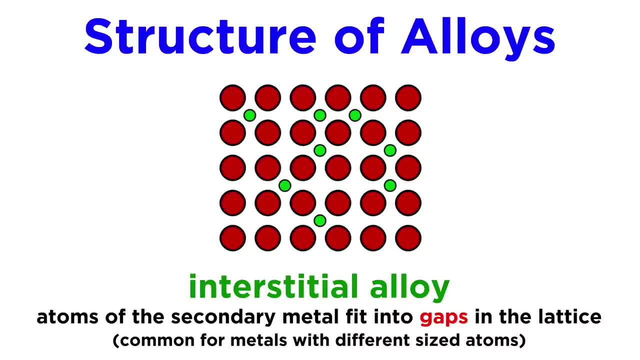 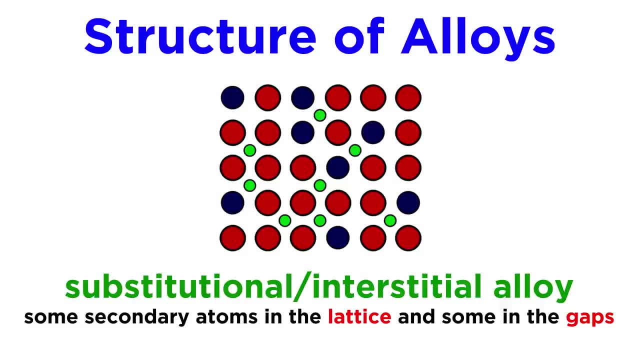 smaller than the atoms of the primary metal, such that they can fit in the empty spaces. And then, finally, there are substitutional interstitial alloys which combine both of these structural features, With some atoms replaced by atoms of the primary metal: the atoms of the interstitial alloy. 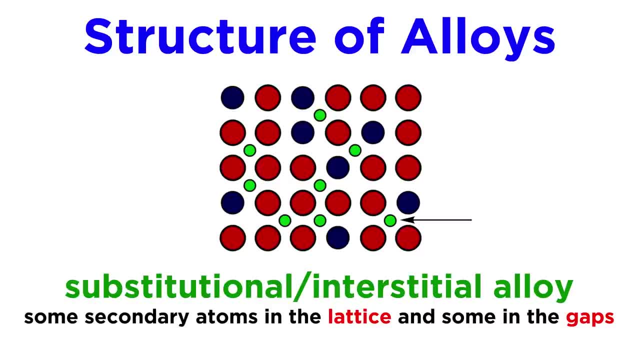 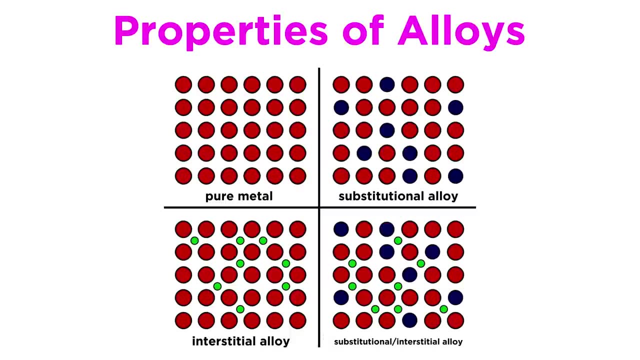 are replaced by atoms of another element and atoms of yet another element found in the interstitial locations. This is quite common for alloys containing three or more metals, as each of them may be of a totally different size. These different structural arrangements can result in different properties for the alloy. 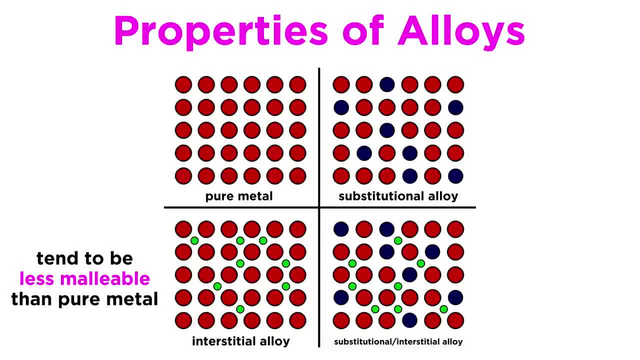 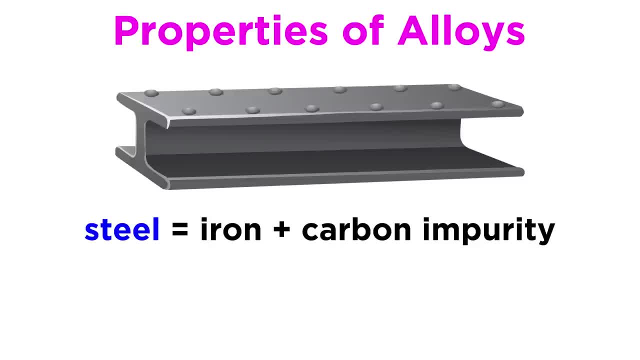 For example, interstitial alloys tend to be less malleable than their pure metal counterparts. Consider steel, which is iron with a carbon impurity. Even though carbon is a non-metal, it can behave like a metal to form an alloy with iron. 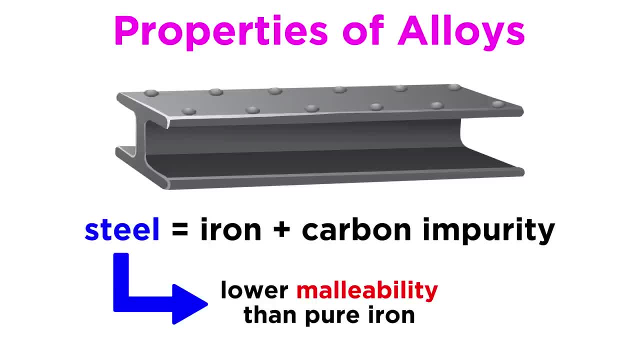 This impurity makes it more difficult for the metal to deform, and thus steel has a much lower malleability than pure iron. This is what makes it such an amazing material for construction. it has a remarkable resistance to compression. There are many kinds of steel that contain trace impurities other than carbon, and each 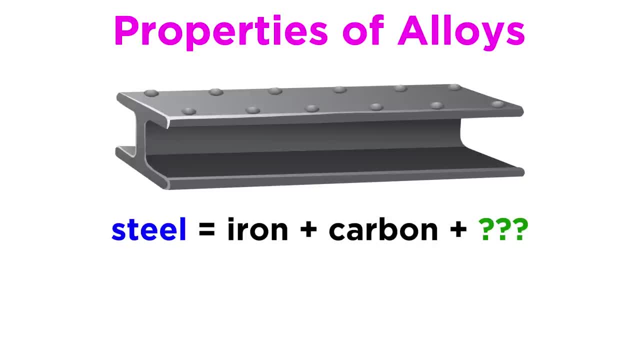 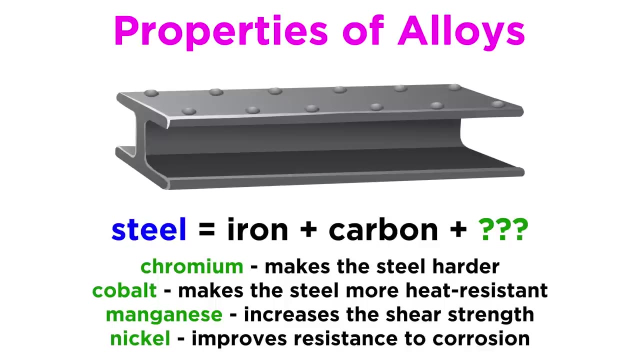 variety has its own, slightly different properties and applications, So let's take a look at some of them. Chromium makes the steel harder, Cobalt makes it more heat-resistant, Manganese increases shear strength, Nickel improves resistance to corrosion, And there are others still.